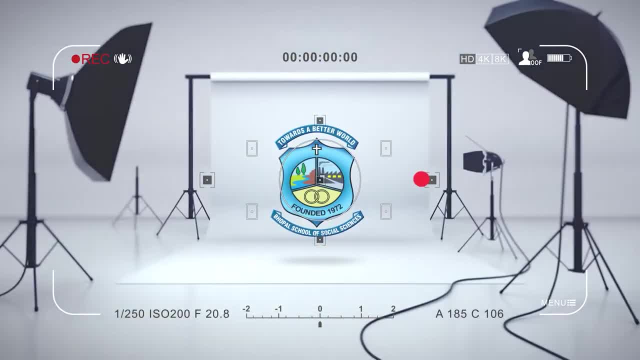 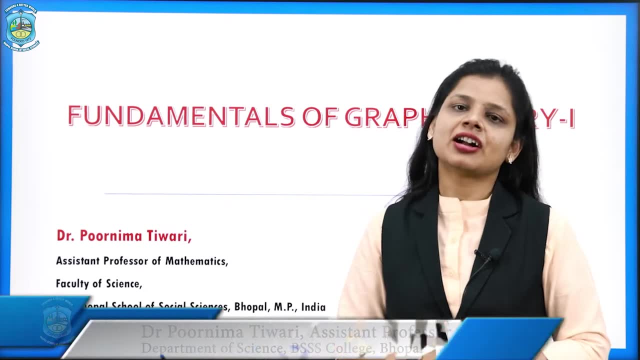 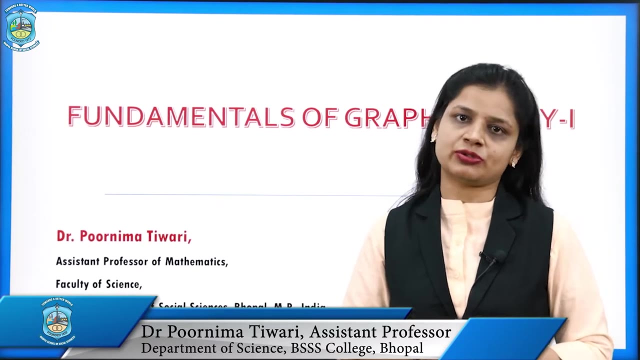 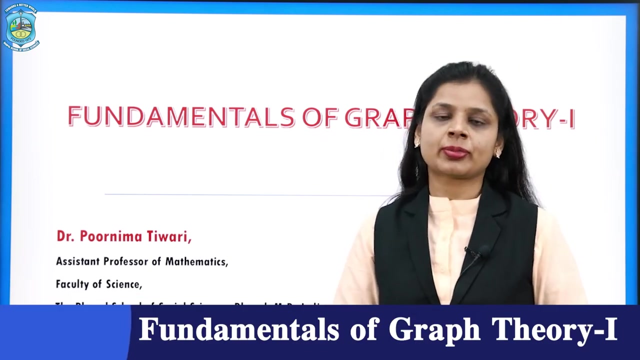 Hello learner, I am Dr Purnima Tiwari, Assistant Professor of Mathematics, Faculty of Science, the Bhopal School of Social Sciences. In this video lecture series, you are going to learn about graph theory. Graph theory is an applied branch of mathematics which has many applications. 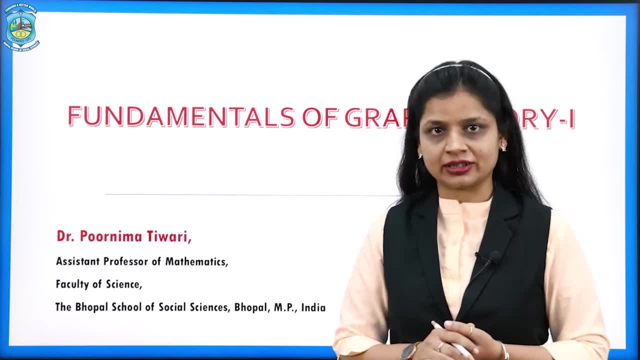 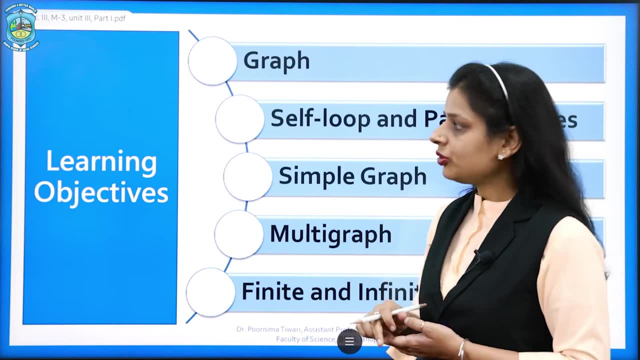 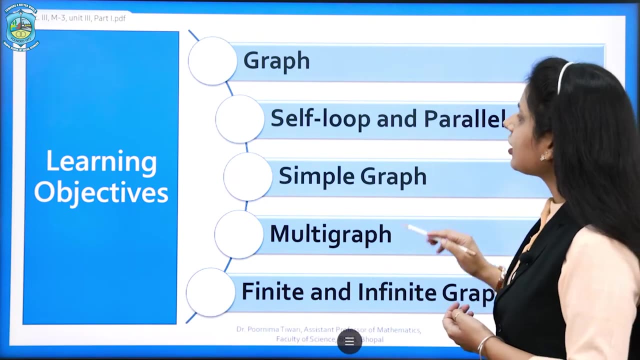 in the field of engineering and computer science. We will start with fundamental concepts of graph theory and in this video you are going to learn about graph, self-loop and parallel edges in a graph, A classification of graph based on self-loop and parallel edges, which are simple graph, and 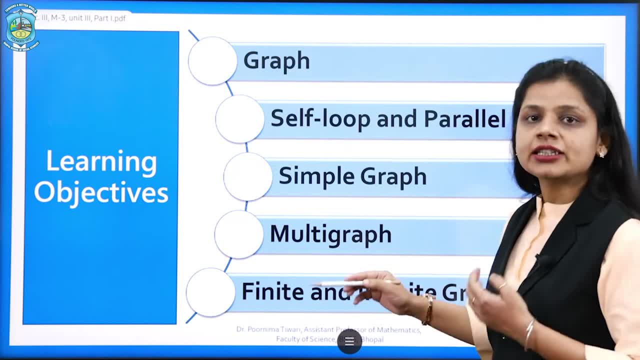 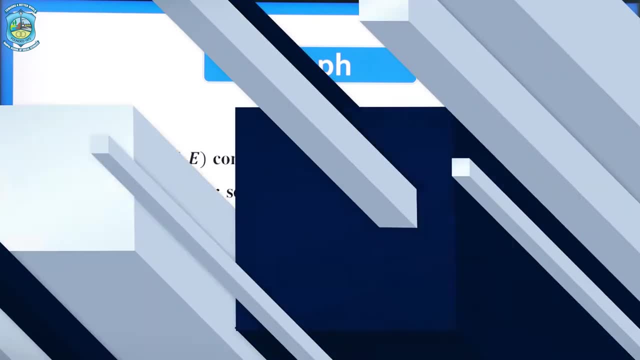 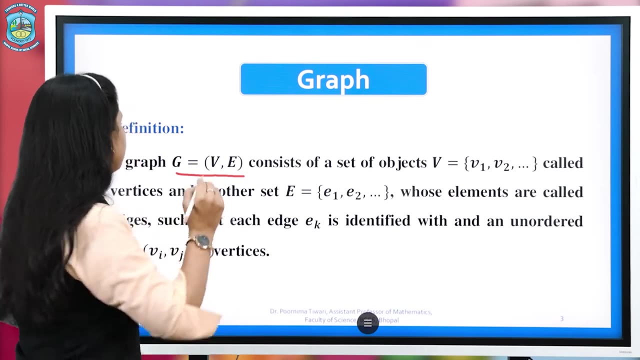 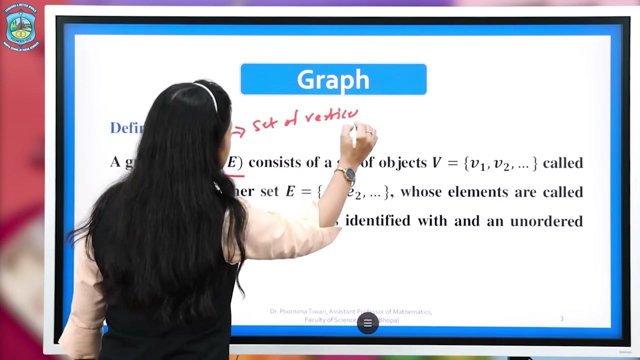 multi-graph. One more classification: finite and infinite graph. Let us start with the definition of graph A graph is represented by g equal to ordered pair of v, e, where this set, v, is set of vertices And another set, e, is set of edges. 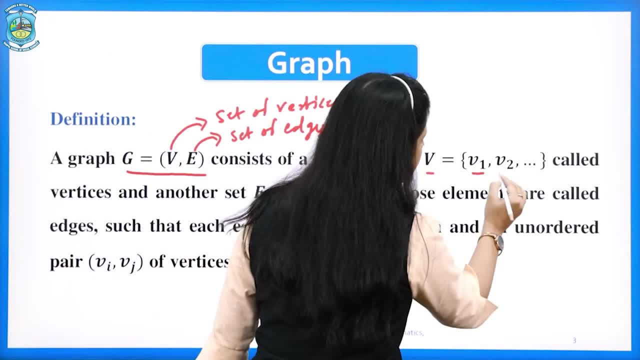 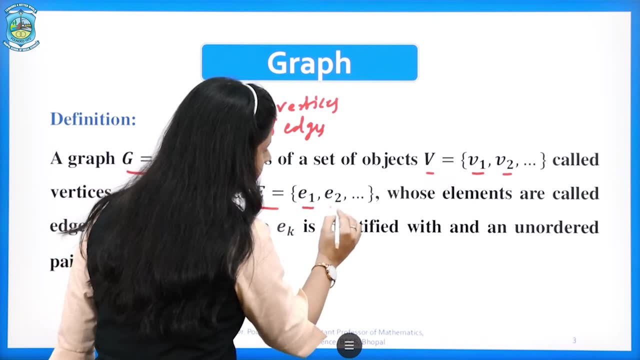 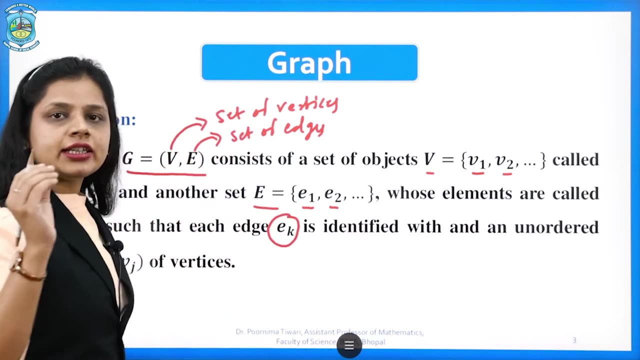 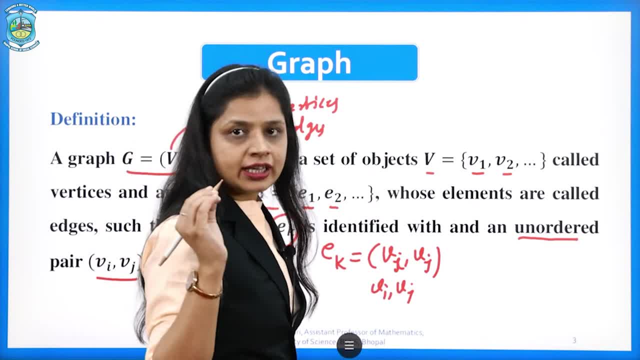 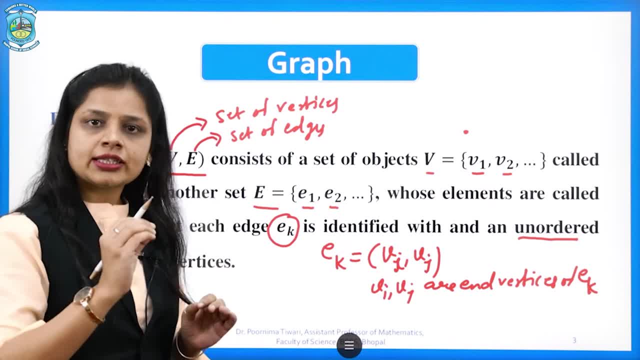 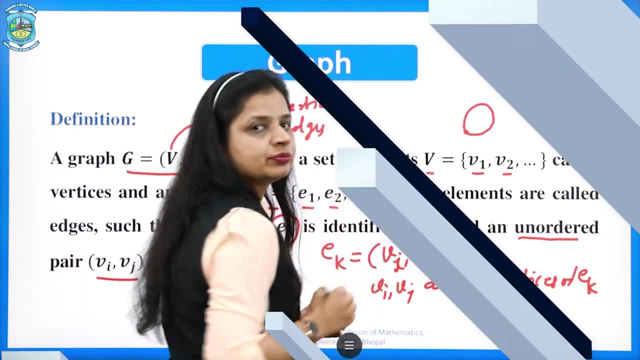 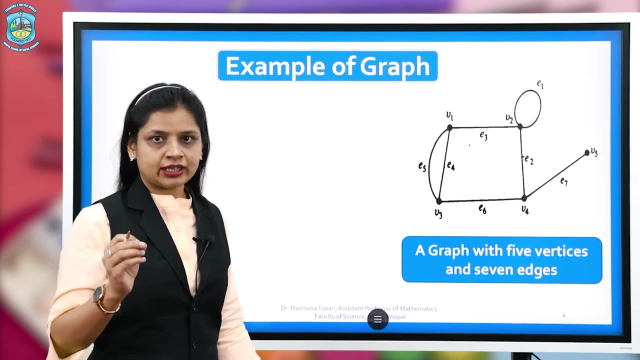 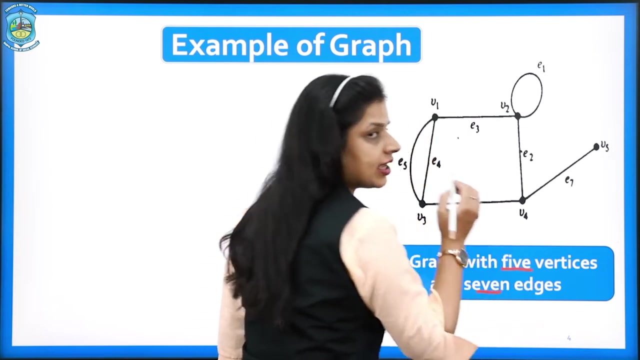 And we can draw this line segment as a straight line or a curved line or in the form of loop. A graph have two types of representation: One in a form of diagram, which is called graphical representation. Now, this is a graph with 5 vertices and 7 edges. 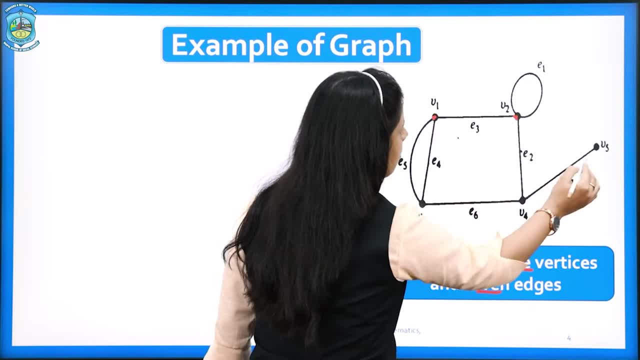 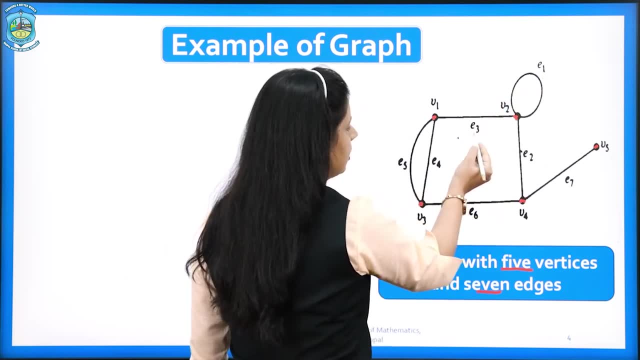 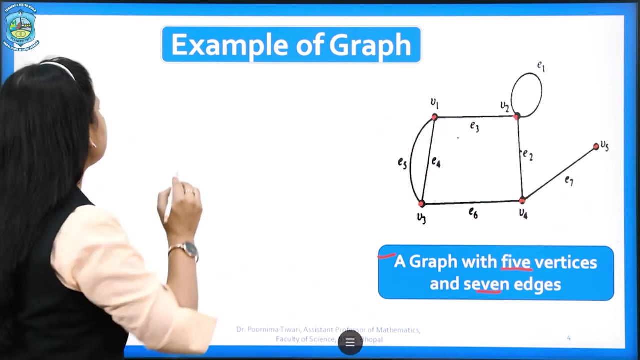 Vertices are V1,, V2,, V3,, V4 and V5, and edges are E1, E2, E3,, E4,, E5, E6 and E7.. When we write this graph, mathematically, we will write it as G, equal to ordered pair of VE. 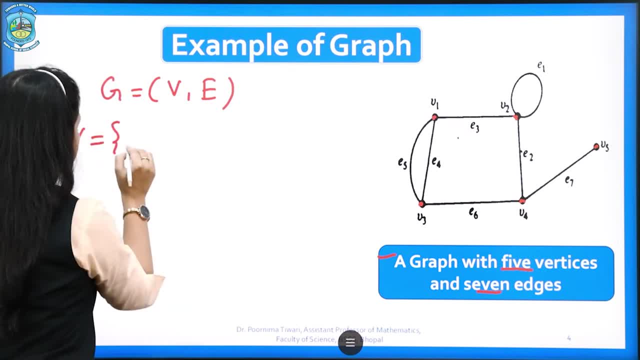 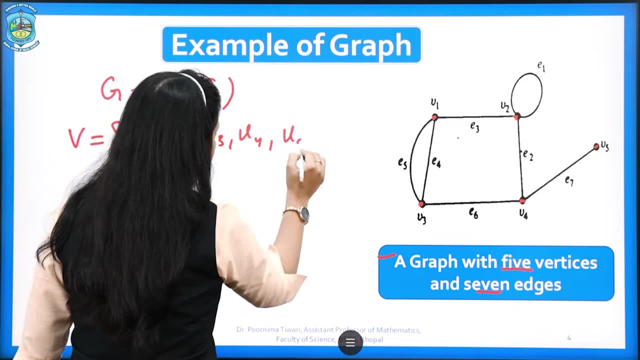 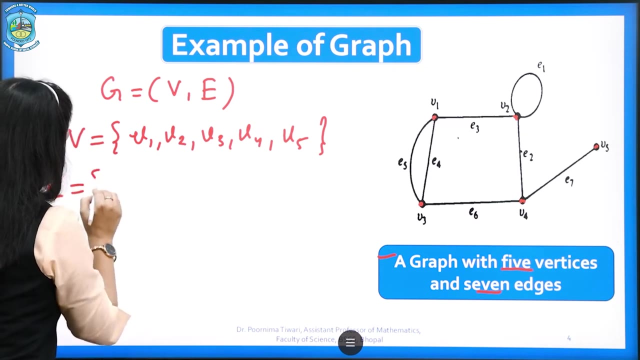 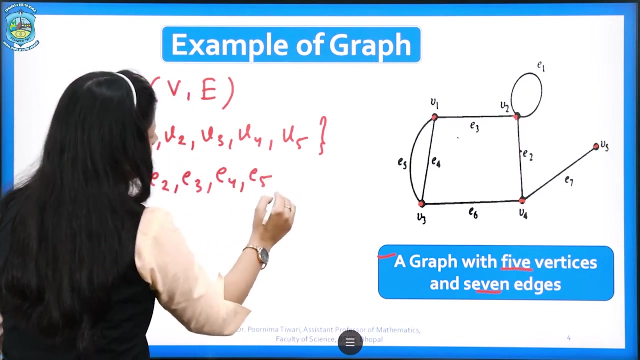 This set of vertices have elements V1.. V2,, V3,, V4 and V5 vertices of this graph Set of edges have elements E1, E2, E3, E4,, E5, E6 and E7.. 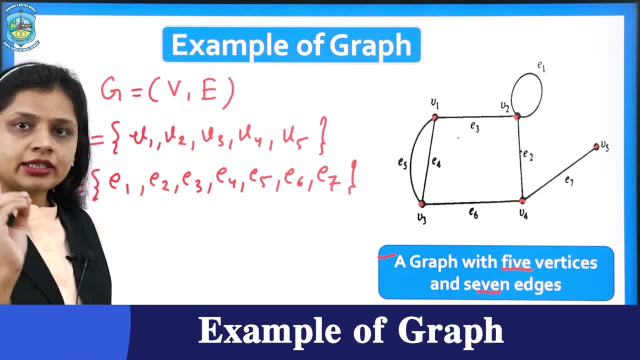 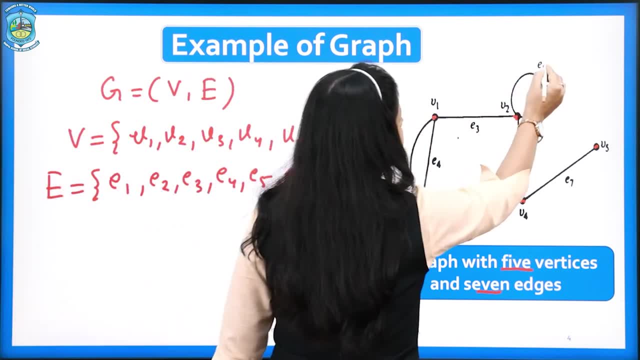 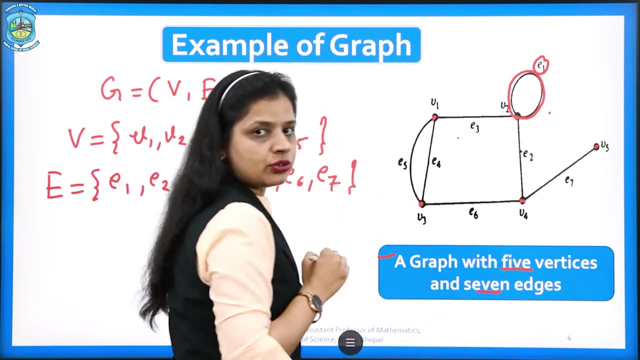 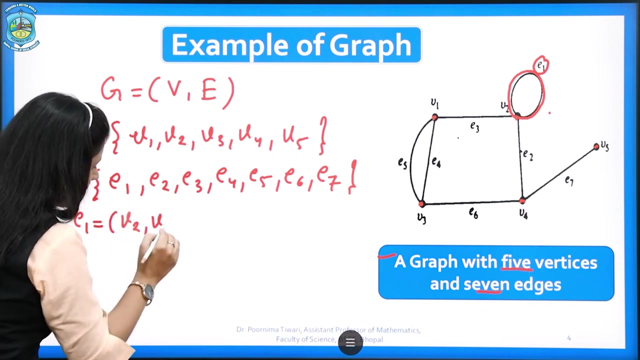 And the condition that each edge identify with a certain unordered pair of edges. We can see this: edge E1 starts with this vertex V2 and ends at the vertex V2.. It means edge E1 is identified by the pair V2 and V2.. 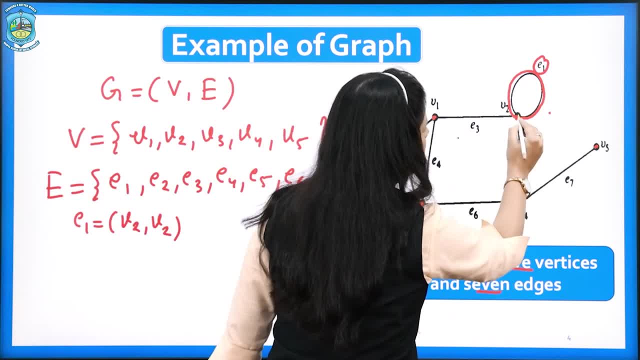 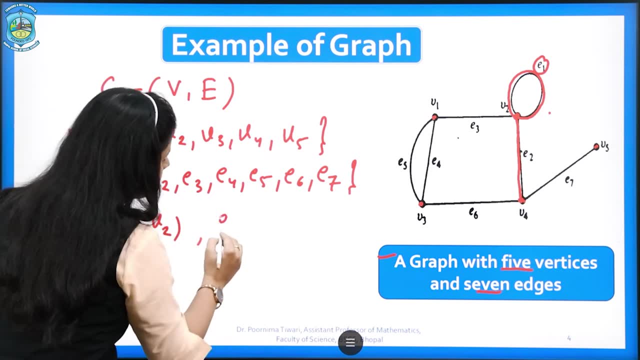 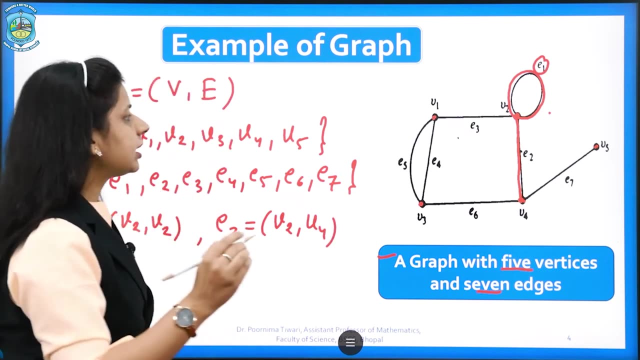 When we talk about this second edge, E2, it lies between vertices V2 and V4. That is, We write edge E2 in between the vertices V2 and V4.. Now, third edge, E3 lies between the vertices V1 and V2.. 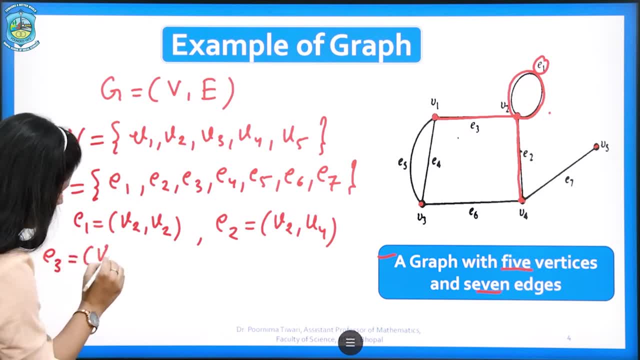 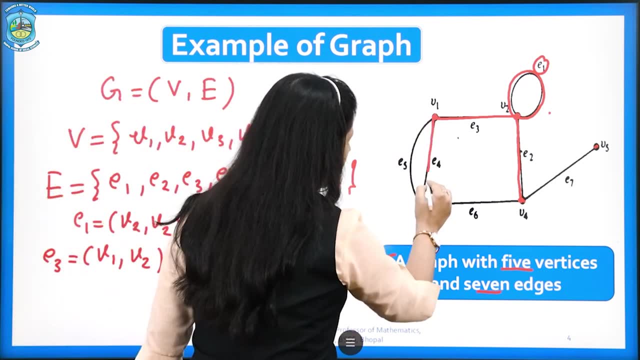 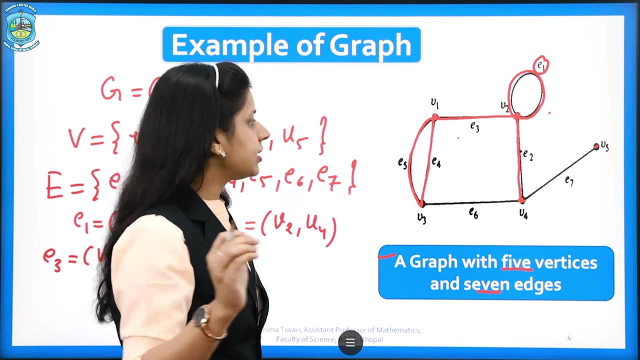 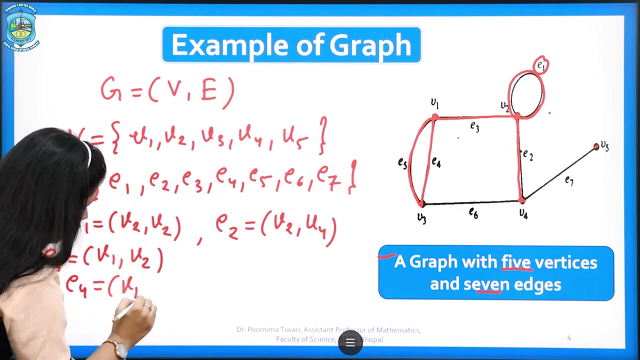 So edge E3 in between the vertices V1 or V2.. When we observe edges E4 and E5. Both edges are identically Identified by vertices V1 and V3. That is E4 in between the vertices V1, V3. 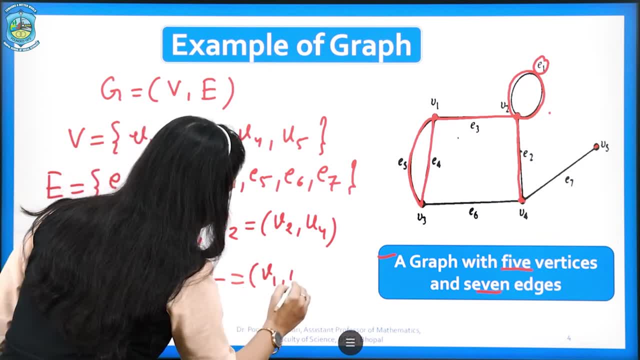 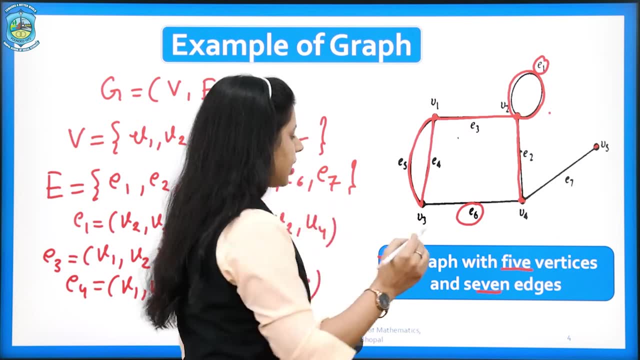 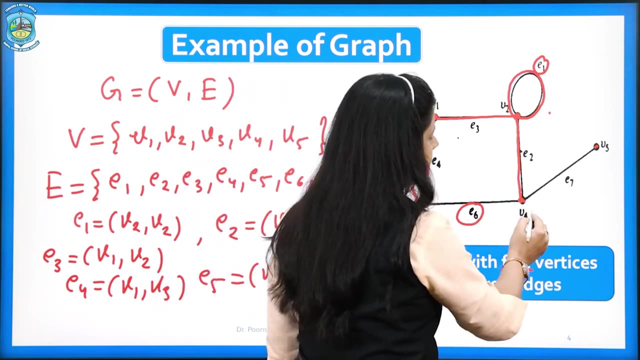 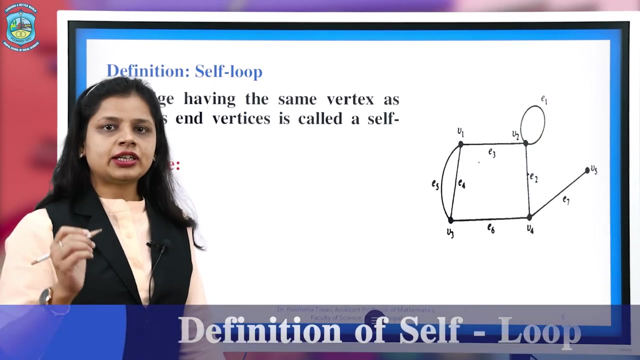 E5 in between the vertices V1, V3.. Likewise, we find edge E6, identified by pair of vertices V3 and V4.. And edge E7, identified by Pair of vertices V4 and V5.. Next definition is self-loop in a graph. 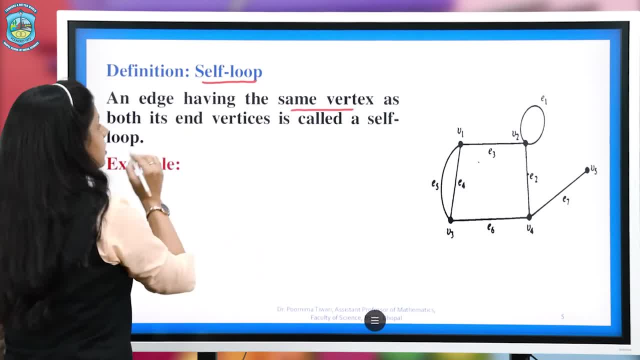 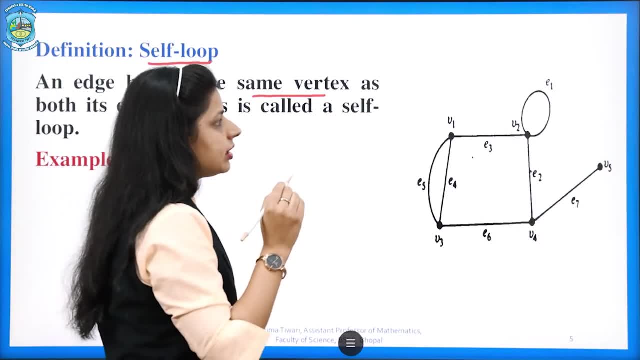 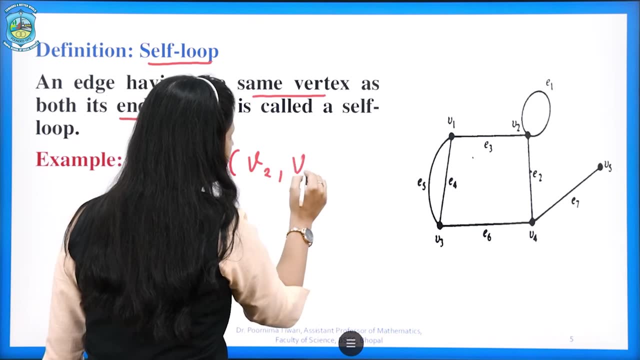 An edge having same vertex as both of its end vertices is called a self-loop. If we observe this graph, we find that this edge E1, identified by pair of vertices V2 and V3.. And edge E7, identified by pair of vertices V2 and V3.. 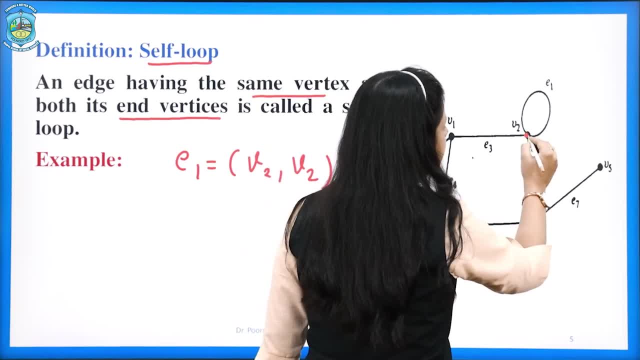 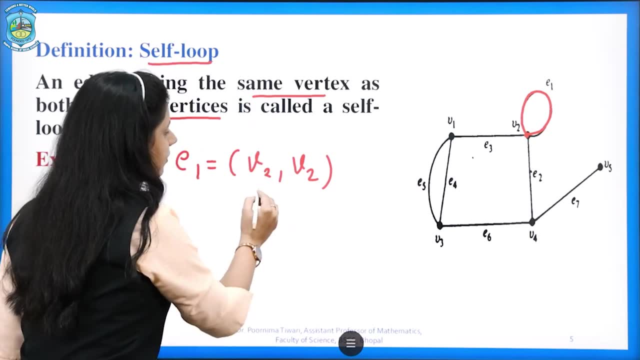 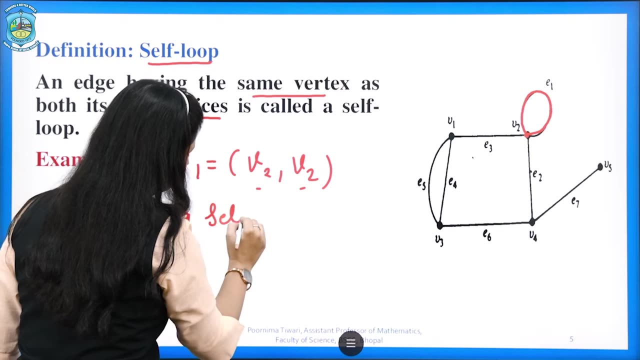 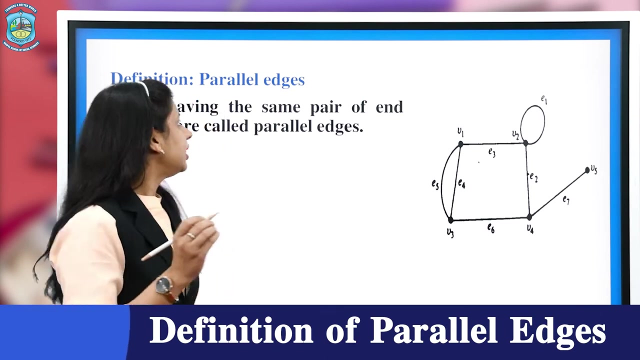 This edge E1 start at the vertex V2.. And starts and ends at vertex V2.. It's both end vertices are the same. So this edge E1 is a self-loop. Next definition is parallel edges in a graph. Next definition is parallel edges in a graph. 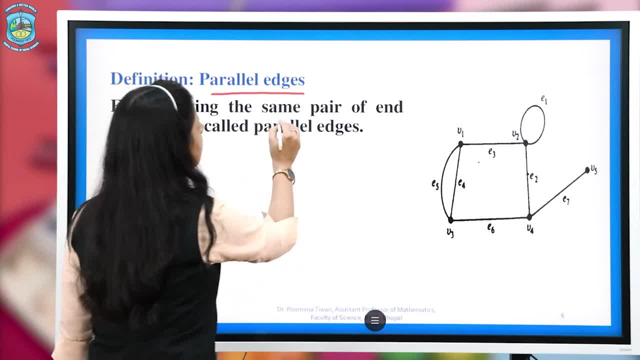 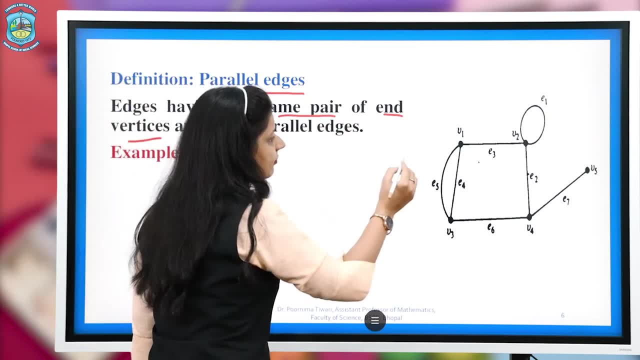 Edge having same vertex. comfort with stylus. Next definition is parallel edges in a graph. Next definition is parallel edges in a graph suggests the even vanilla values like the same ancestry. there again, there pair of end vertices are called parallel edges. If we observe this graph we find that edge. 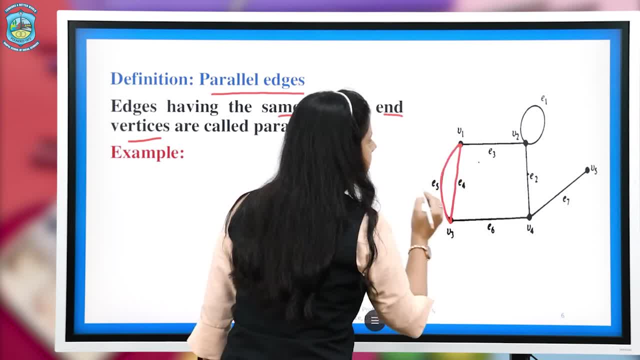 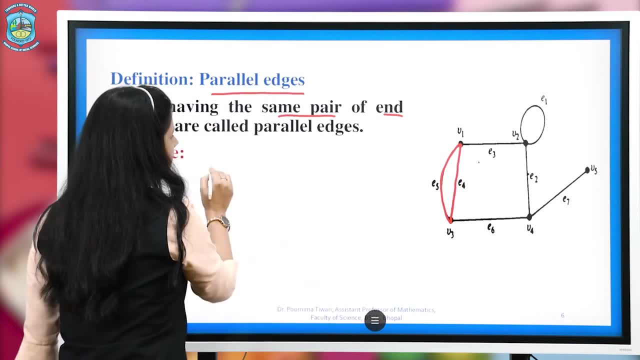 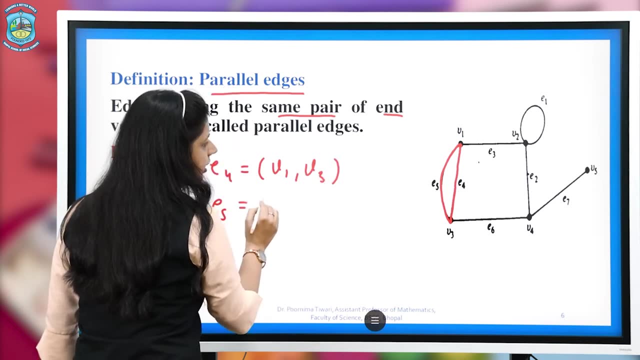 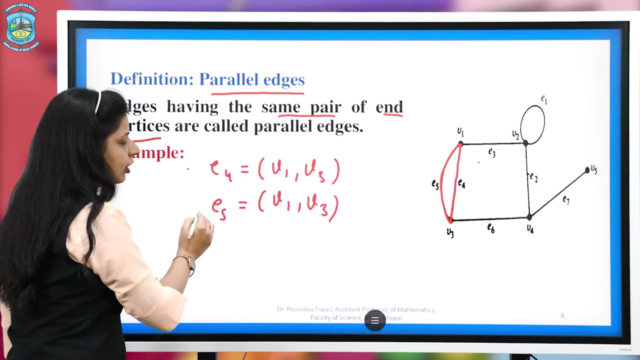 E4 and edge E5, identified by pair of vertices: V1 and V3.. So edge E4 lies between the vertices V1, V3.. Edge E5 lies between the vertices V1, V3.. Edges E4 and E5, both identified by same pair. 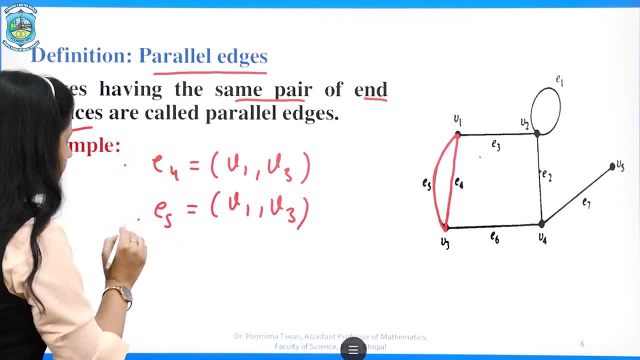 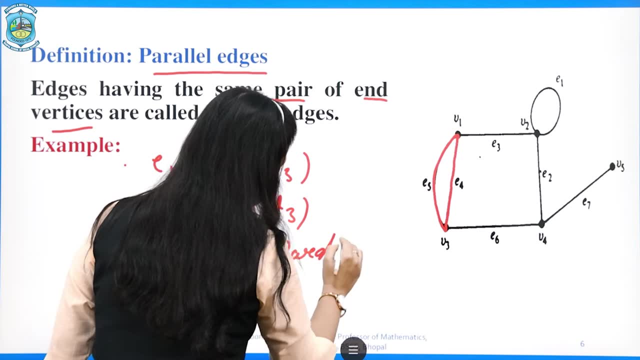 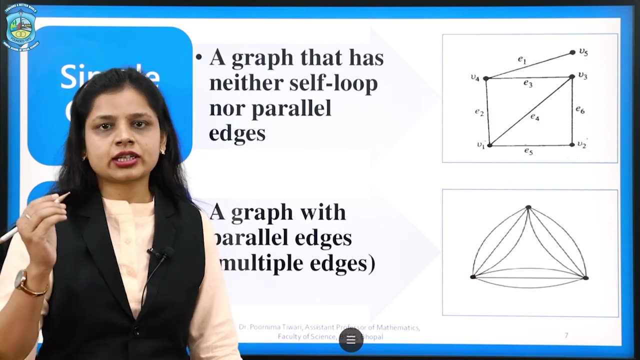 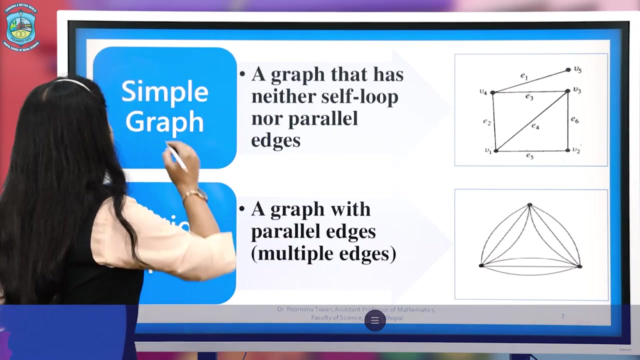 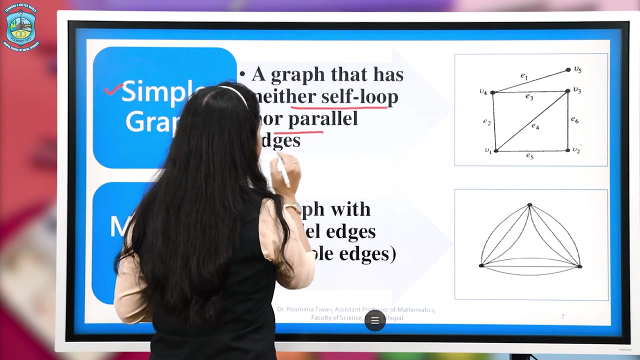 of end vertices V1 and V3. Therefore, E4 and E5 are parallel edges. Next we will discuss classification of graph based on the property, self-loop and parallel edges. First is simple graph. A graph that has neither self-loop nor parallel edges is called. 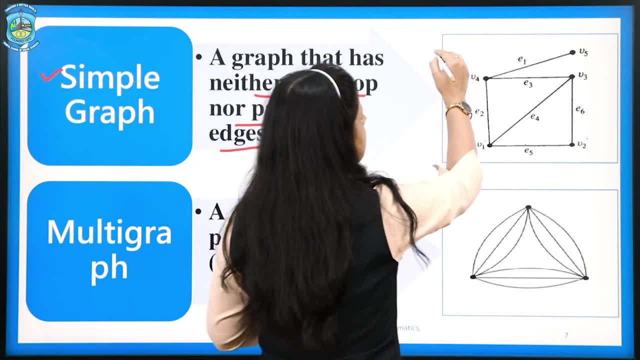 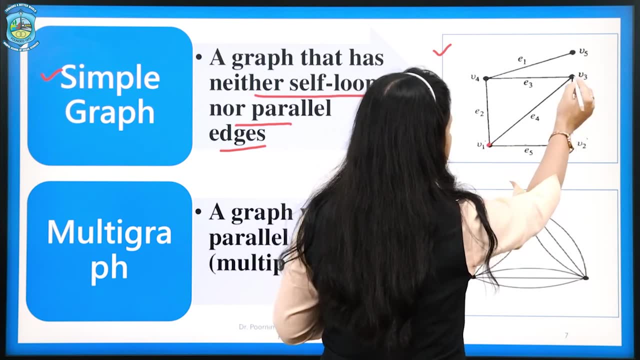 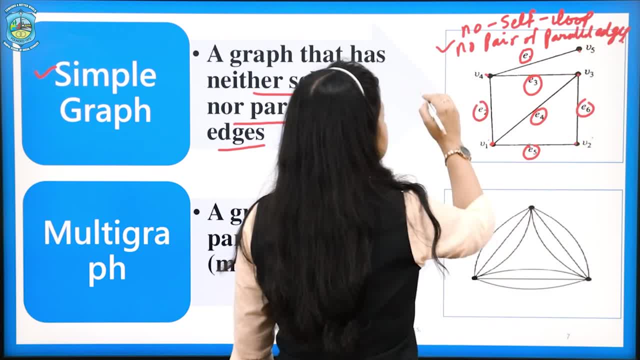 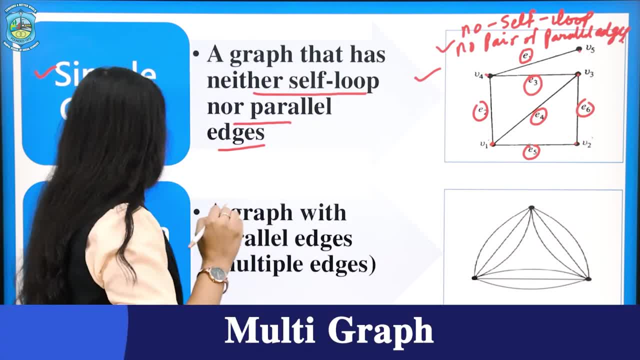 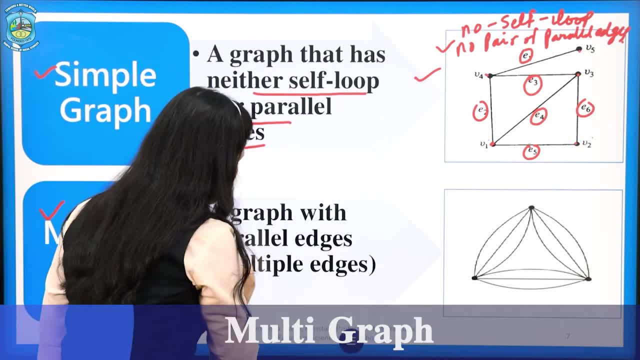 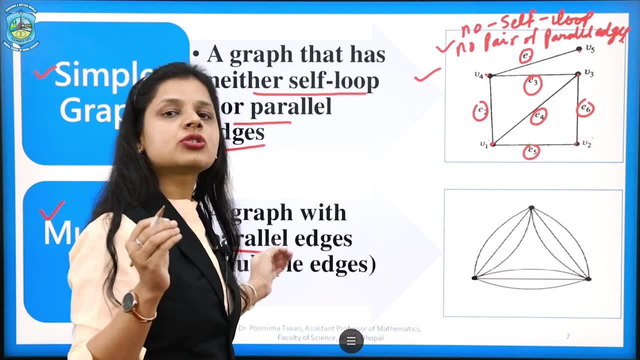 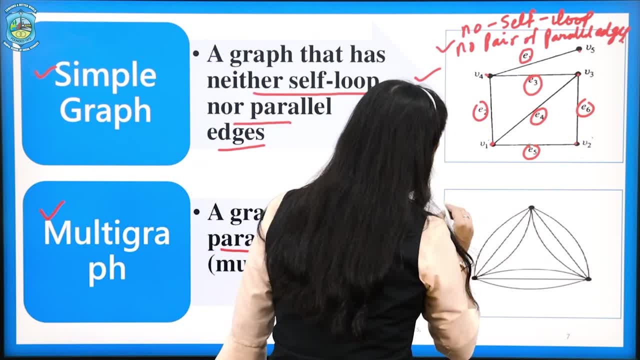 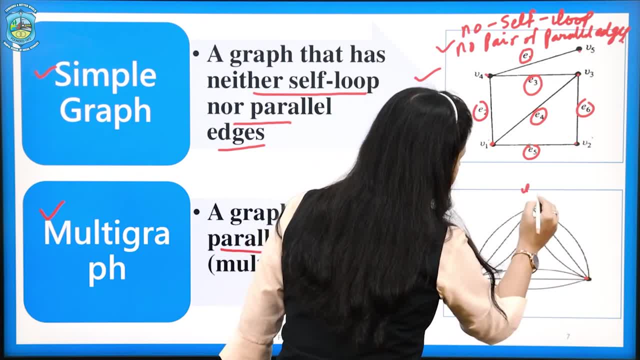 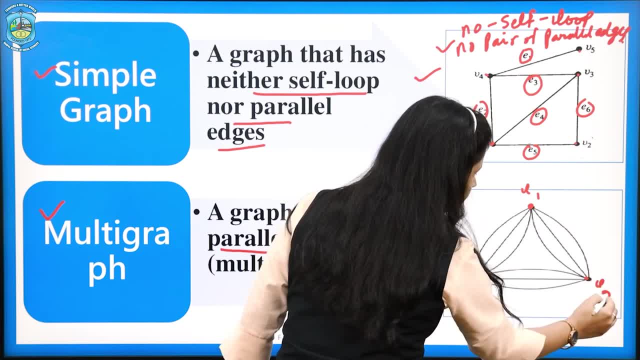 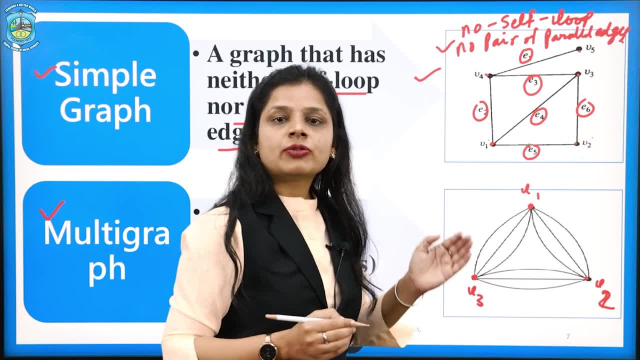 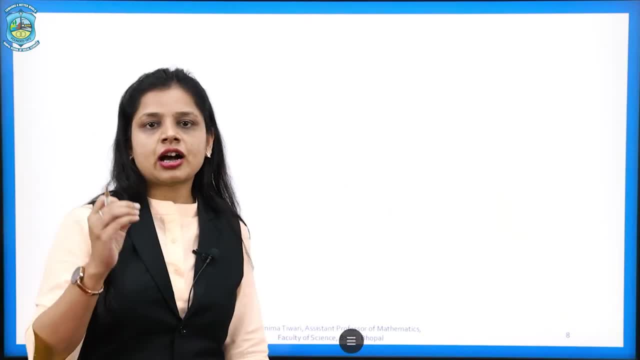 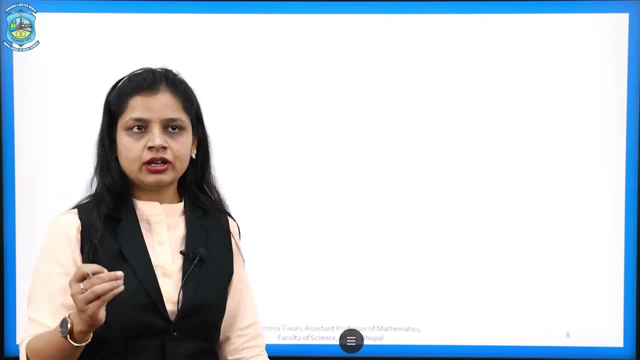 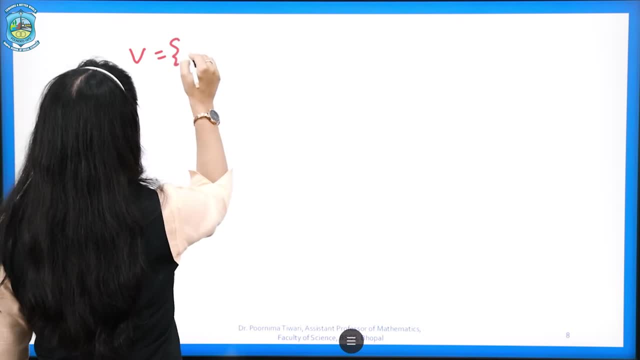 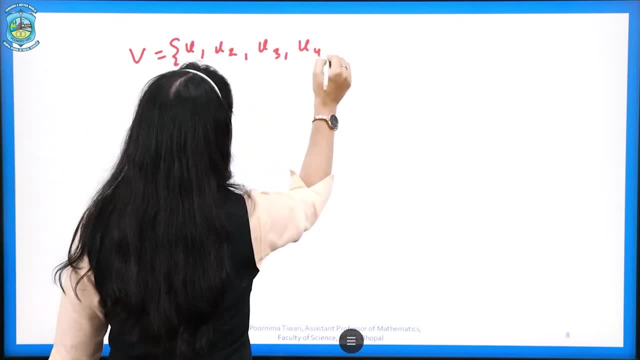 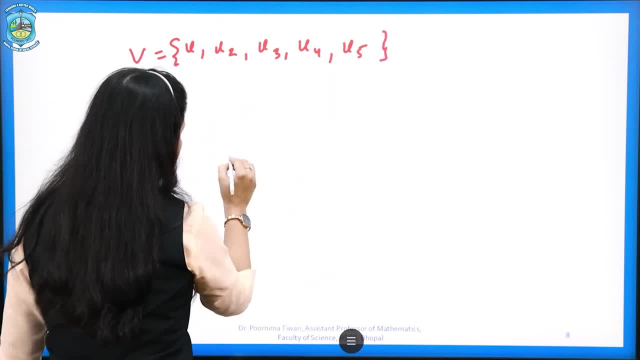 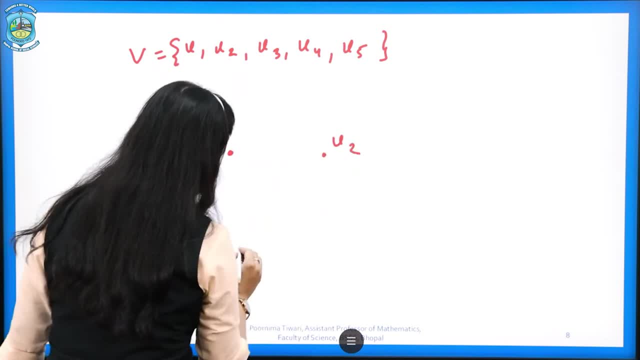 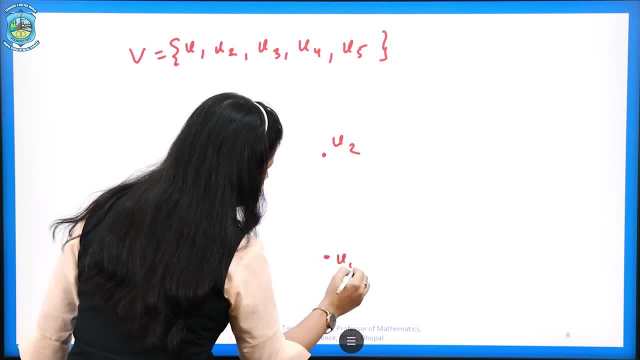 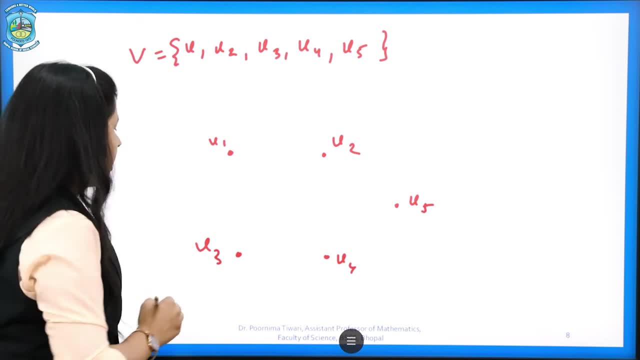 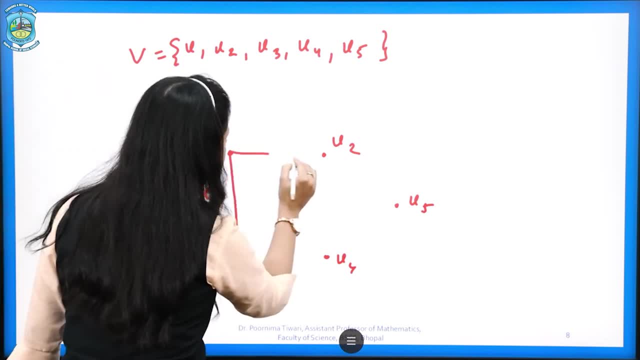 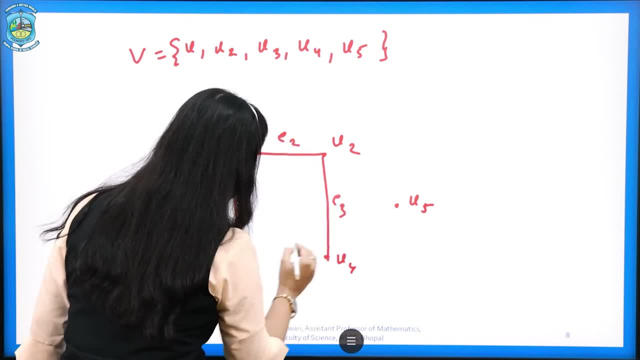 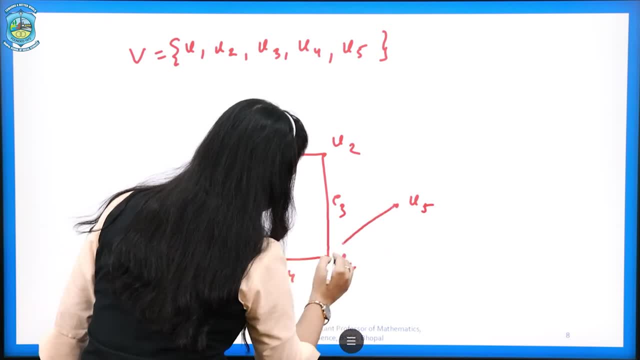 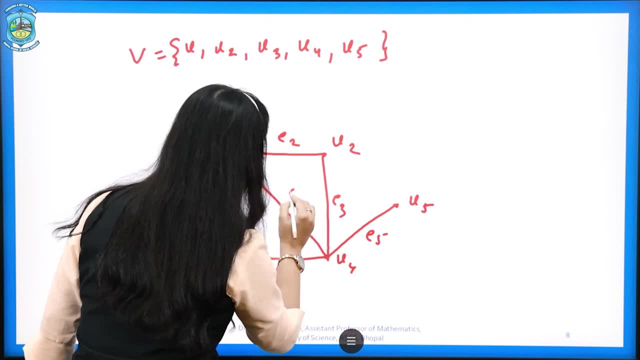 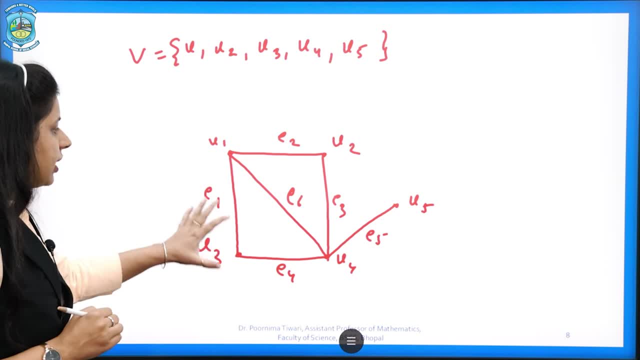 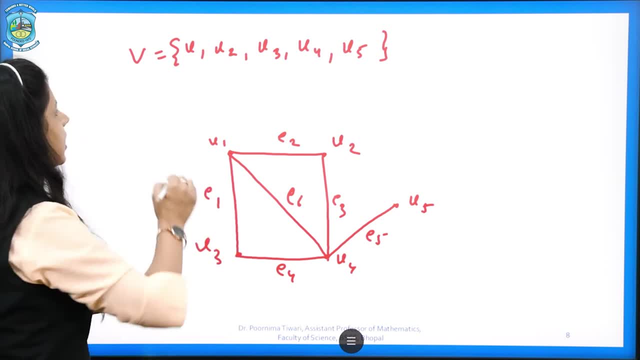 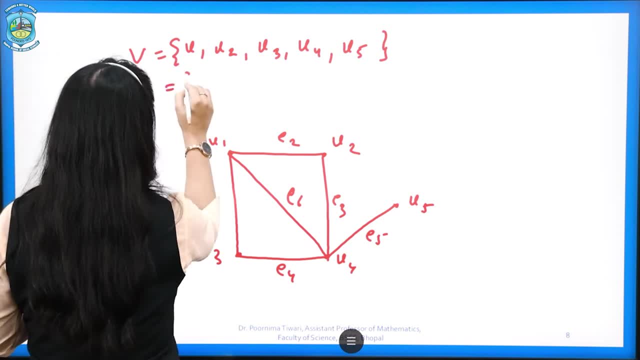 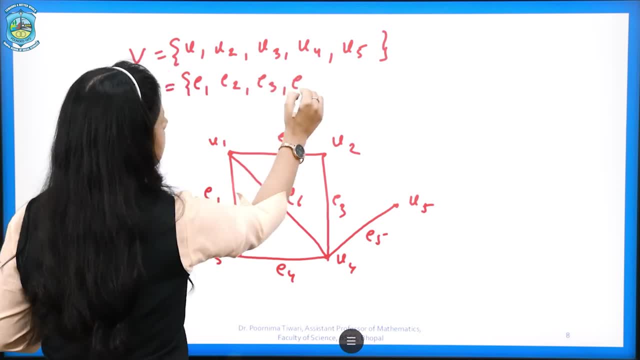 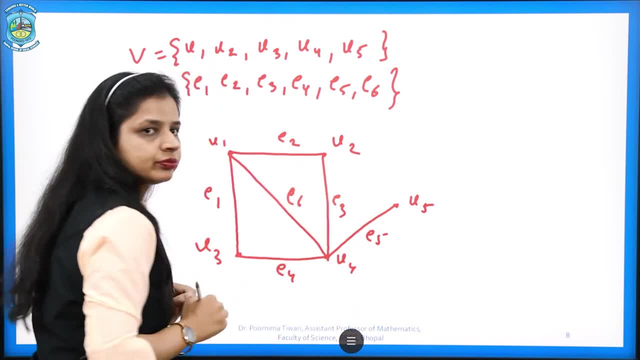 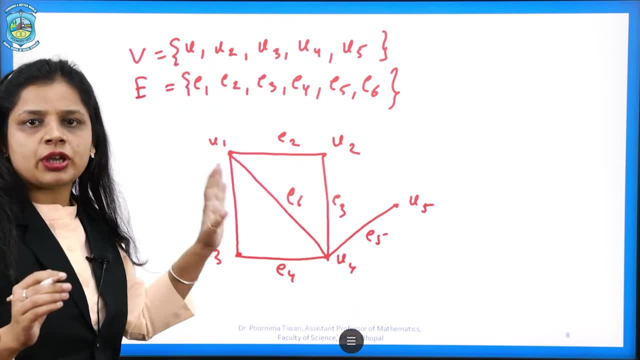 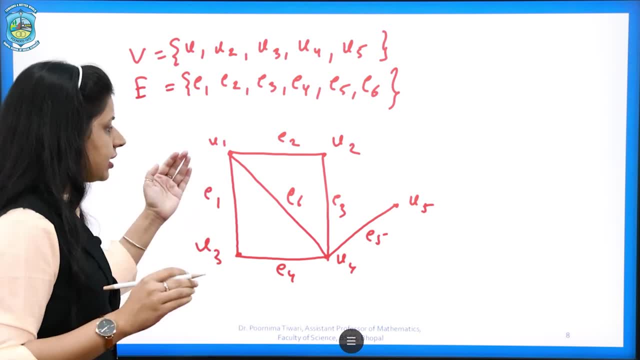 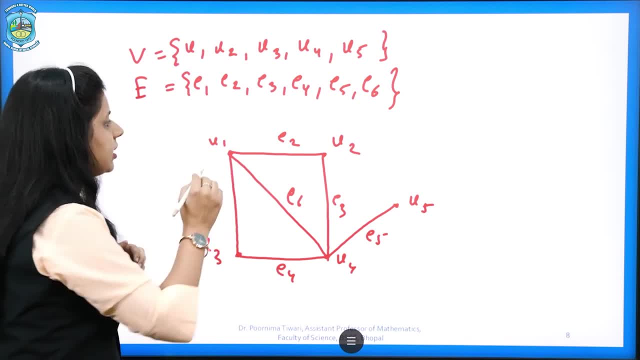 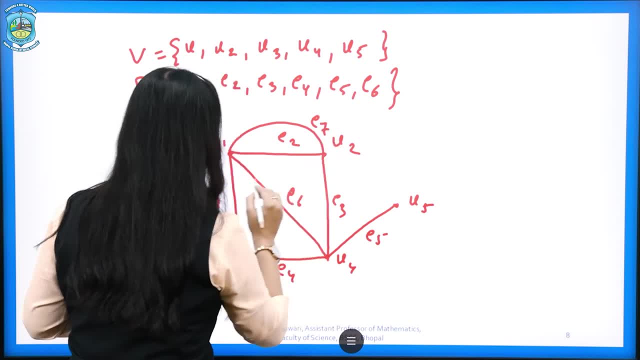 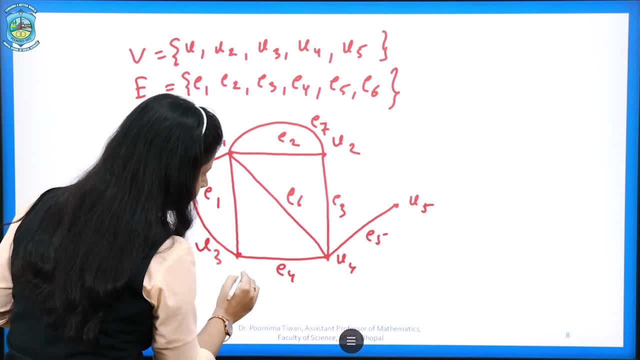 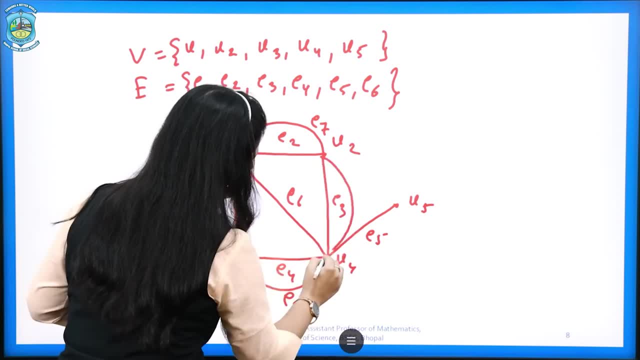 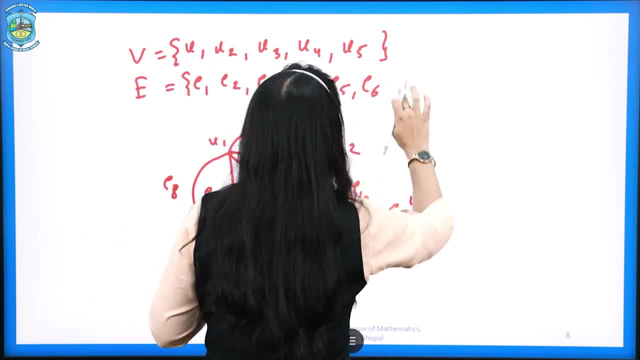 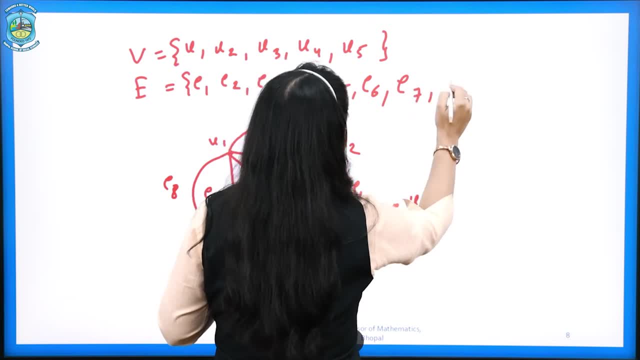 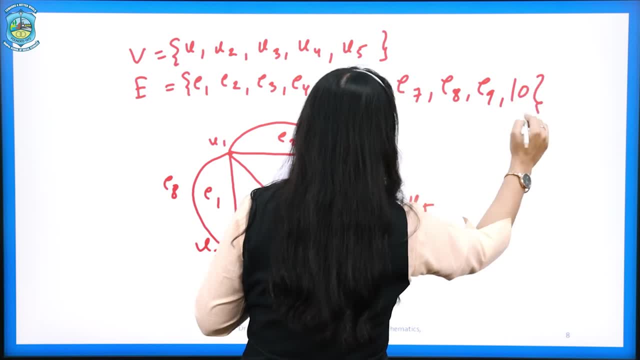 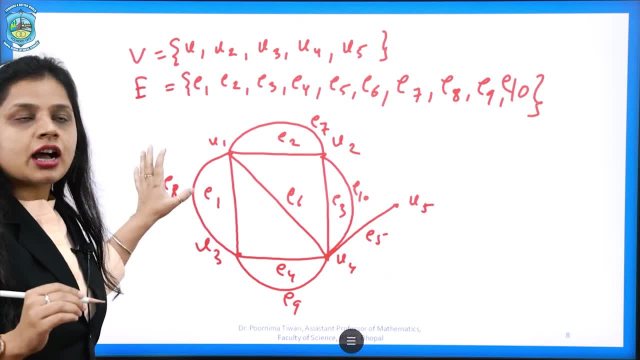 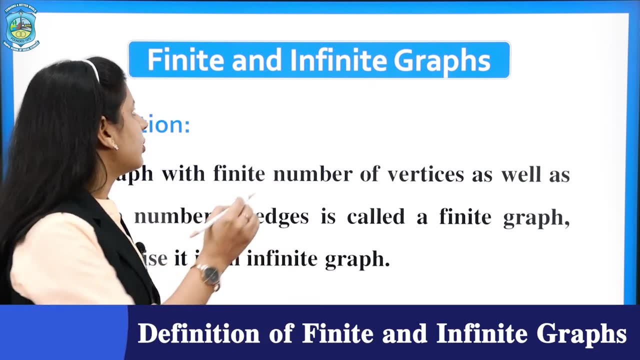 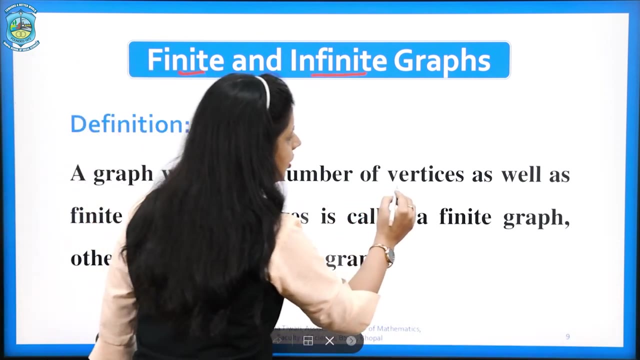 So this is a simple graph. So this is a simple graph, So this is a multigraph with 5 vertices and ten edges. Next definition is for finite and infinite graph. A graph which has finite number of vertices as well as finite number of edges is called.